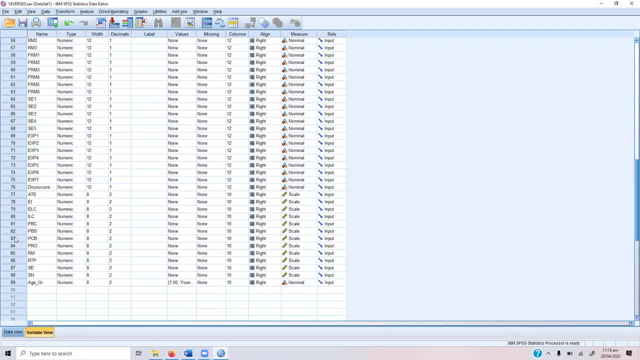 So I've already created or transformed this variable into a single measure, a PCB, And I want to evaluate whether PCB differs between male and female respondents or their perception of contextual barriers actually differs between male and female respondents. But the problem is that I've identified that the PCB variable is non-normal. 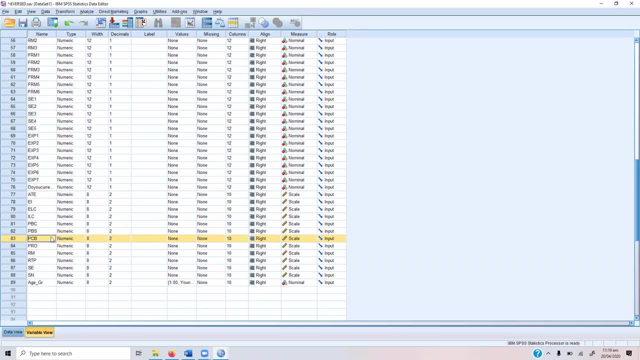 So how would I check for differences between male and female if I've got data which is non-normal? So a simple and easy way to do this is you use non-parametric tests. So go to analyze non-parametric tests and in the legacy dialogs you use two independent samples. 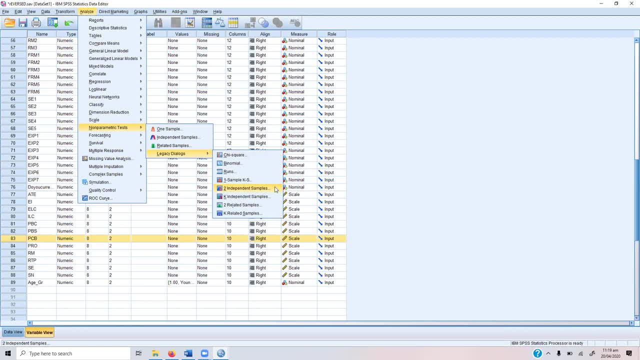 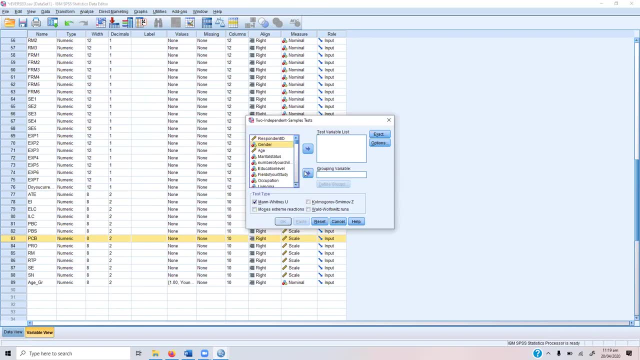 Because you've got two independent samples, One is male, the other is female. You just test this- two independent samples- And you select your categorical variable in which you want to evaluate. And you select your categorical variable in which you want to evaluate. 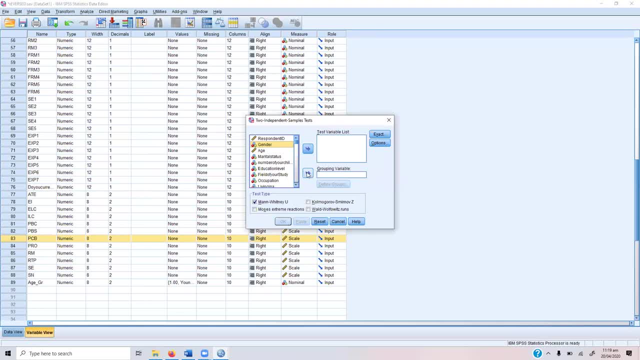 And you select your categorical variable in which you want to evaluate. want to evaluate the differences. in this case, we want to evaluate whether perceived contextual barriers, or the perception about the contextual barriers, actually differs between male and female respondents. so you select your categorical variable, press this arrow button right before. 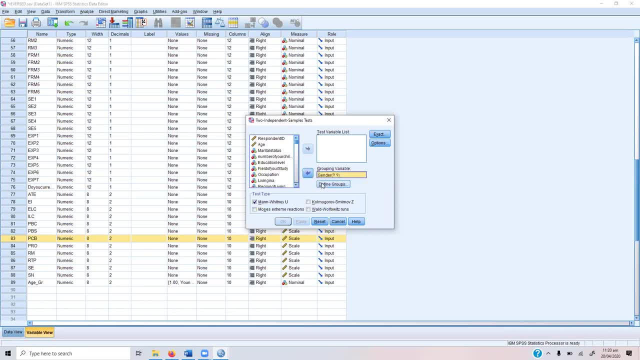 this grouping variable and you define your groups. in this case we have got two groups identified by one and two. you press continue and i am interested in perceived contextual barriers. so this is what i want to test, so you can test multiple variables, and then man whitney, you test is selected. 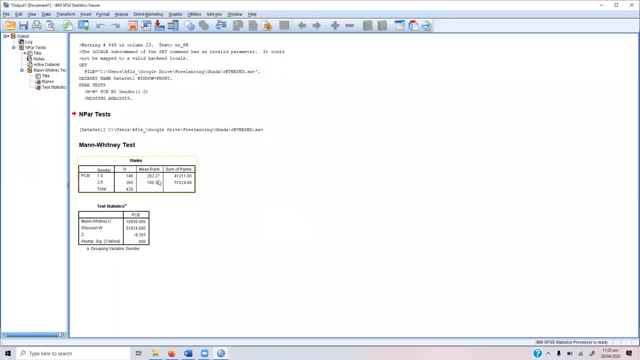 so you just press ok and here are the results. so, if you see, there is mean rank or sum of ranks, there is n and then there are the two categorical variables and what we are interested in is this, and in test statistics, statistics, we are interested in significance. so if we look at this significance, this is less than 0.05. so this means that there are 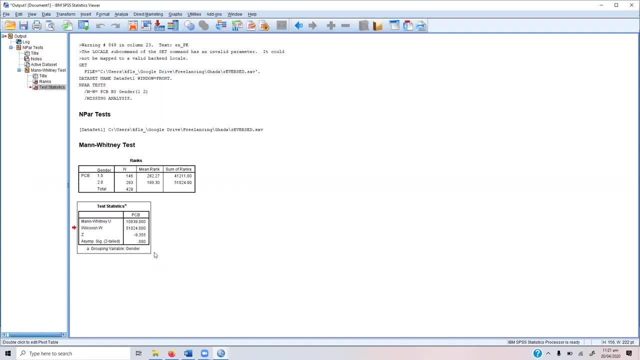 significant differences in the perception about contextual barriers between male and female respondents. so the way that male employees think about contextual barriers is different in comparison to females. now if you see that the mean rank it's 282 and the mean rank for females is 180.. now this means that the perception about contextual barriers 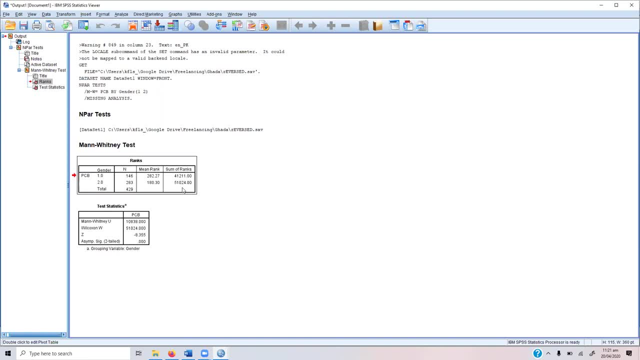 is high that this means that male perceive that the contextual barriers are higher in comparison to females. so a higher mean rank in this case means that, according to males, in their perception the contextual barriers are significantly higher in comparison to females. so females think that the contextual barriers are not that high. so this is one example that one can use. let me run this. 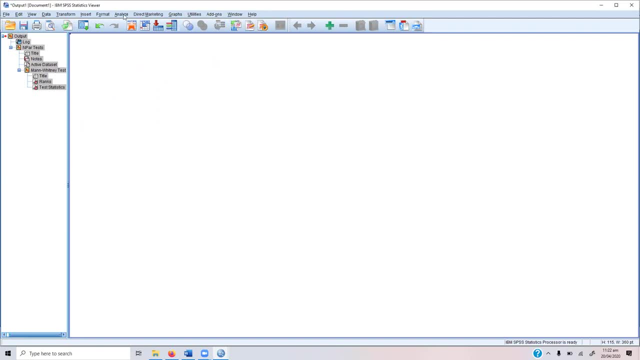 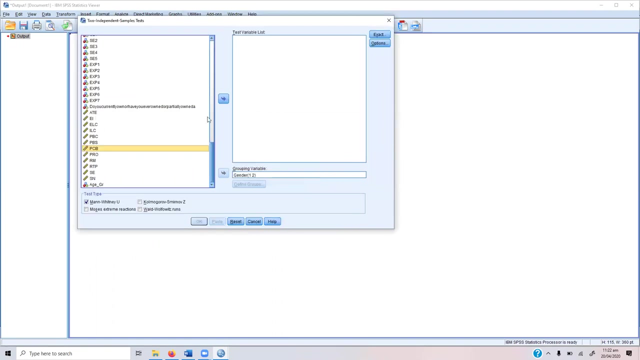 test on the female also. let's see how it works. now we'll update her to the intent test. she will tricky, so let's rescue her from yahoo and use dress code for this case. we're using dress code which Scroll Lag, which has zero 열. 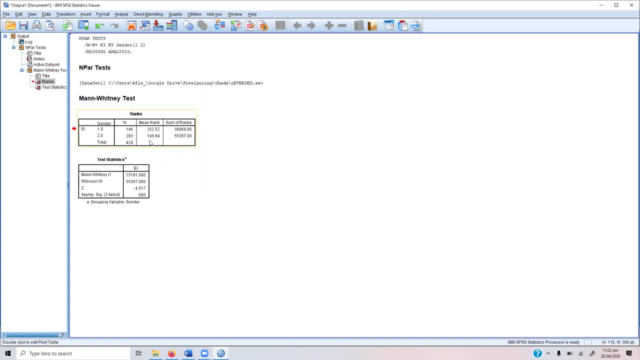 male in comparison to females. so male have got higher entrepreneurial orientation in comparison to female, because the mean rank for male is higher in comparison to females. so what if we want to? and is this difference significant? yes, this difference is significant because the significance value is less than 0.05. now, how would you interpret this? results? just copy these two. 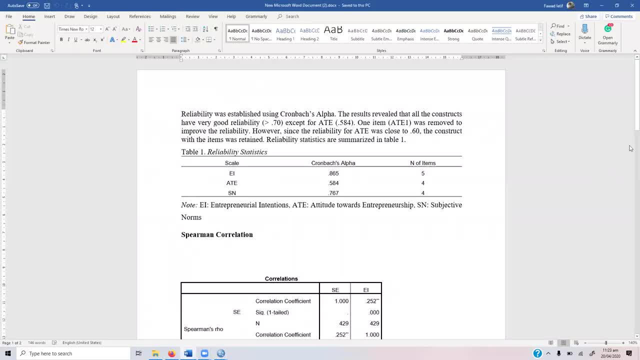 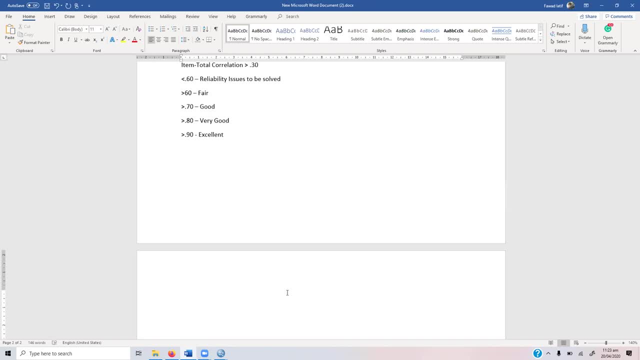 tables and let's get to our document. and if we can just first, okay, let's say, let's, let's first propose our hypothesis that we want to test. so at one is: there is a significant difference in entrepreneurial intentions between male and male respondents. now let's, we've got the results. 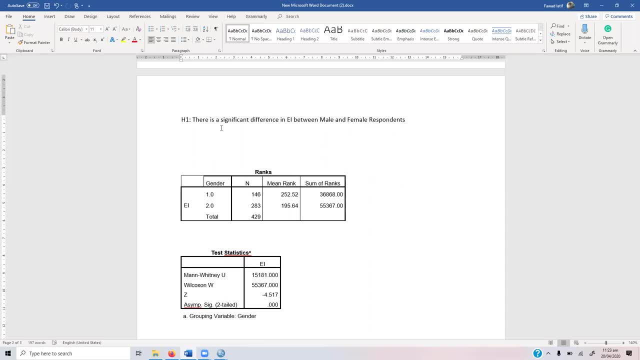 let's interpret and report the results of this hypothesis now. hello, hello, yes, hello. turn off your mics, please. thank you, okay, now let's interpret this. okay, you, So here is your man, Whitney, you statistic, So just you just put it in, and then your. 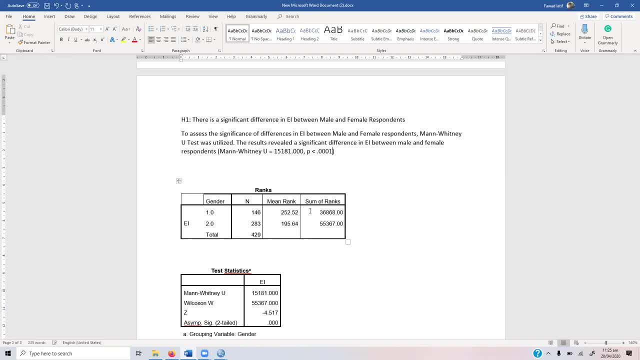 p-value is less than 0.001.. So if it's, if the significance value is 0.000, you just write p is less than 0.001.. Otherwise you just write the p-value as is. p is equal to say if it, if it was. 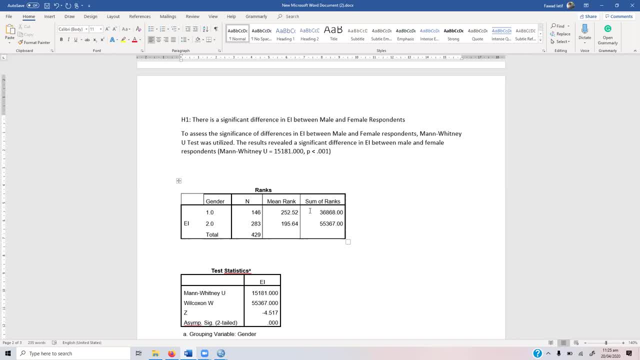 0.10,, 0.010, you would have written: p is equal to 0.010.. You only use the lesser sign when it is 0.000.. 0.010.. Now this is how you actually interpret the results for your man, Whitney. Now, how do you? 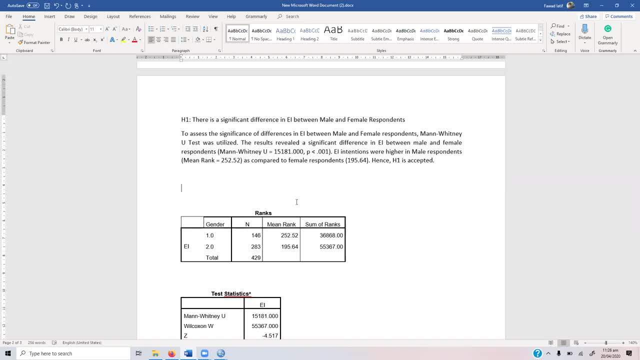 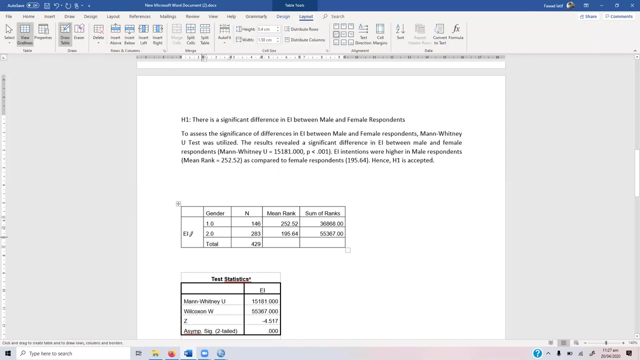 report. You just can't just put these tables in your document. This is against formatting. So what you can do is: let's do this. So you first move this column, you make sure that all borders are highlighted. Let's say I'm going to layout or table. 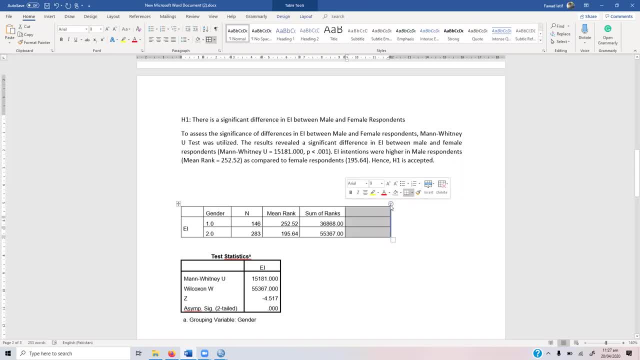 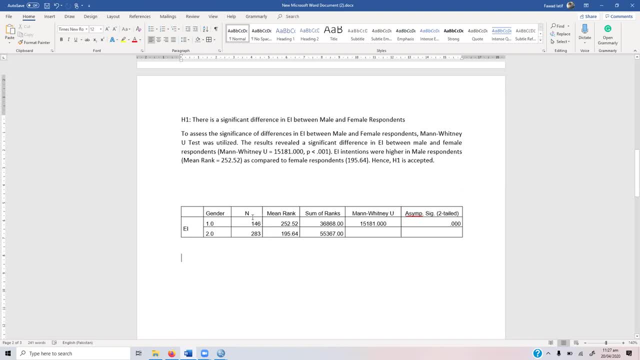 And let's format it a bit, Okay, Okay, Okay, Sorry, I'm a little fussy about this formatting and obviously it's good that one should learn about these formatting as well. Select the bottom border. select the top border and then the first row. just select the bottom. 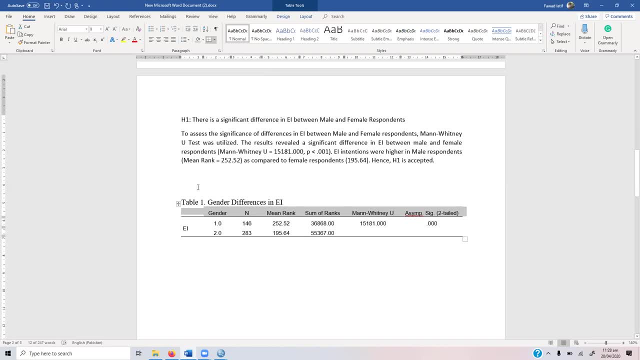 border. Now this is how you can. oh sorry, I might have made a mistake here. So you select the top. Now this is how you report man Whitney uTest in proper now. this is. this is done for man. 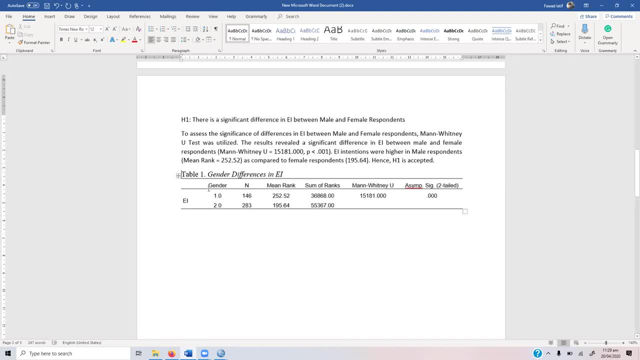 Whitney uTest. If you've got any questions, please ask. Hello, Hello, Hello, Hello, Hello, Hello, Hello. Yes, Any questions? No questions, Okay, Okay, let's go to our final topic. ah, no, sorry, ah, we use, we were to do regression. 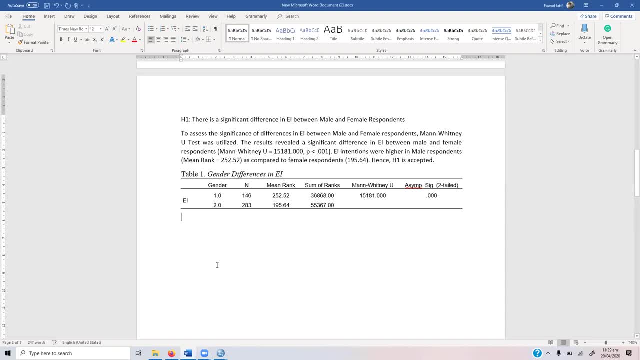 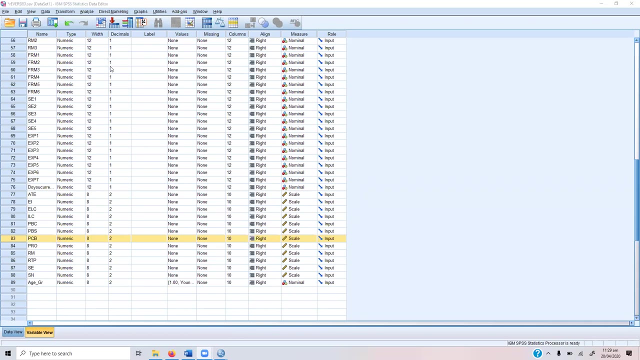 as well. Okay, let's do regression in the end, but now let's keep the theme of differentiation and let's focus on our next test, Ah, which is it's called Wallace Edge Test. Now, in this particular example that we just did, 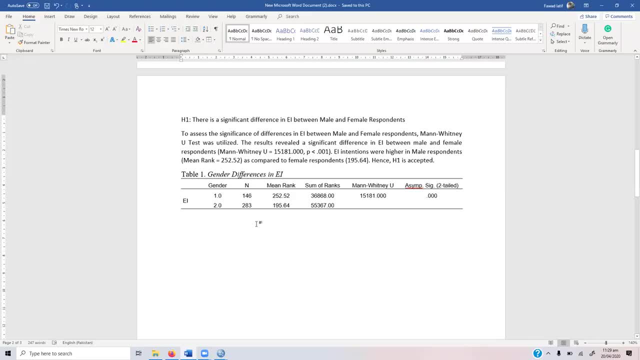 in this example we had two groups, So I wanted to evaluate whether entrepreneurial intentions differ between male and female. What if I've got more than two groups So you cannot use man-between-you test? What if the data is not normally distributed or data is in ordinal scale? 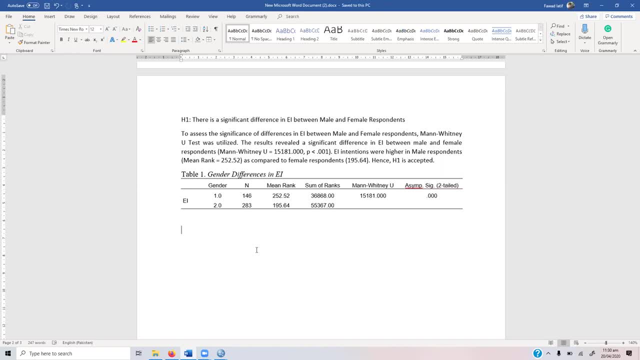 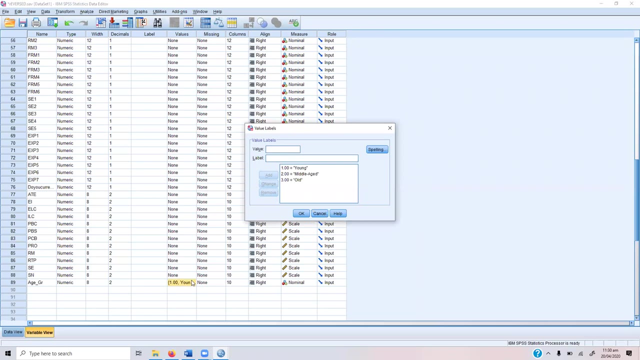 Or at ordinal level, And I'm interested in identifying or evaluating whether a particular variable differs between more than two groups, And in this case, let's say, our groups are maybe age. So I've divided age into young, middle-aged and old. 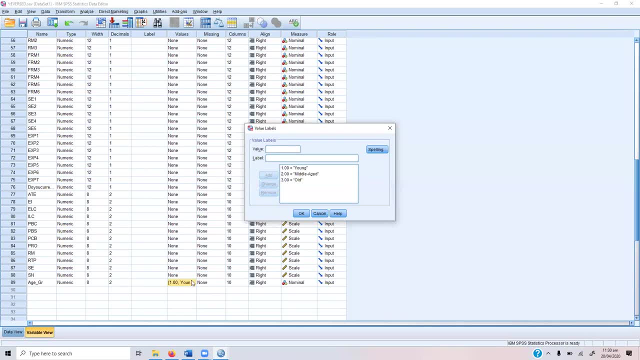 And I want to assess whether entrepreneurial intentions differ between young, middle-aged and old people or not. So how would I conduct a test that would tell me that there are more than two groups, Or how would I conduct a test that evaluates these differences between these three categories? 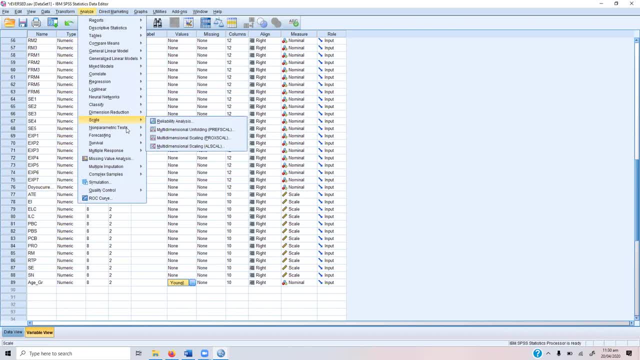 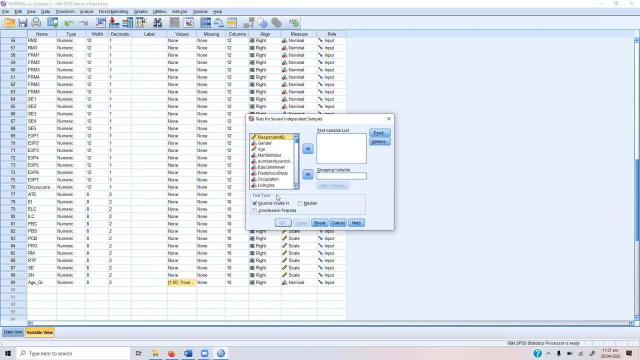 Now, in order to do this, you press Analyze, same non-parametric tests, Legacy, Dialog and K-Independent Samples. So you press K-Independent Samples And I'm interested in age. Define the range. The minimum is one. 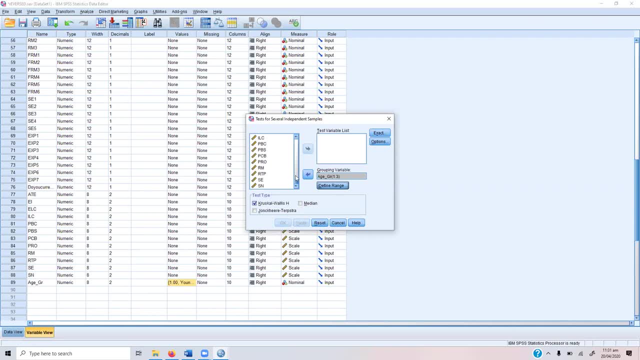 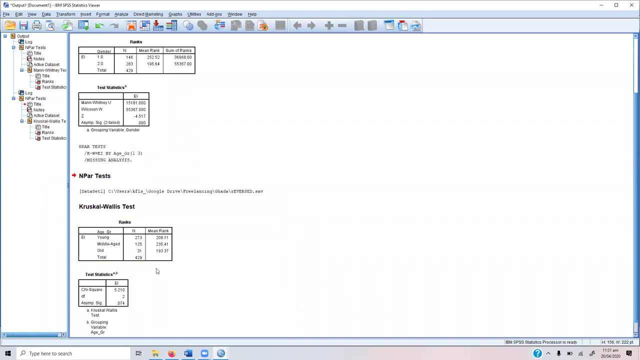 The maximum is three And I'm interested in entrepreneurial intentions. So you select this And Kruskal-Wallis edge test And then just press OK, It will give you the results. Yes, please. Minimum and maximum range is constant, one and three. 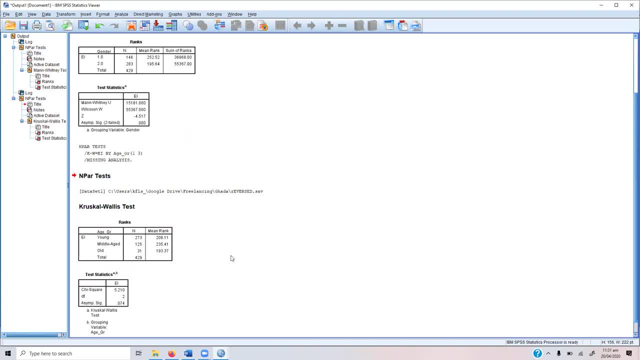 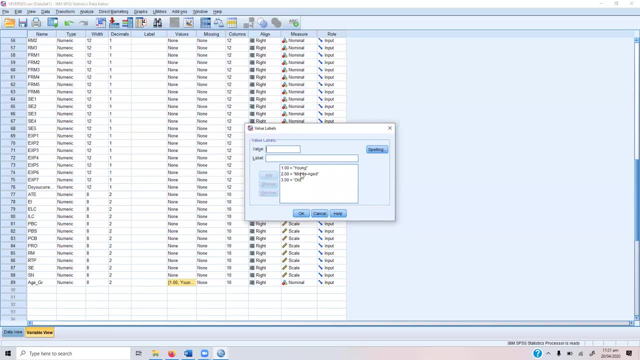 Yeah, because there are three groups. If you see the dialog box on your screen, there are three groups: Young, Middle-aged and old. So one signifies young and three signifies old. So that's why the minimum was one and maximum was three. 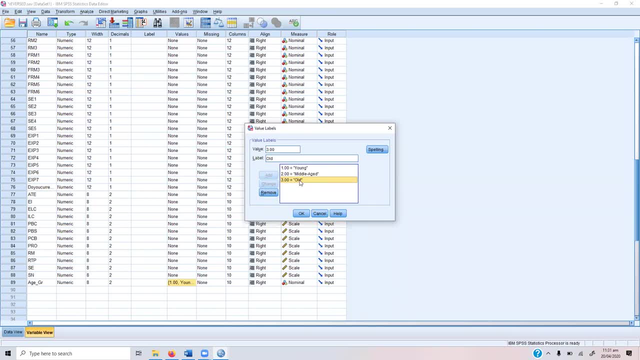 So it's the numeric representation that you have given to your groups. That's why, in our previous session, we mentioned that always try to represent your data in the form of numbers, So this helps you do your analysis. So in this case, I represented young with one, middle-aged with two and old with three. 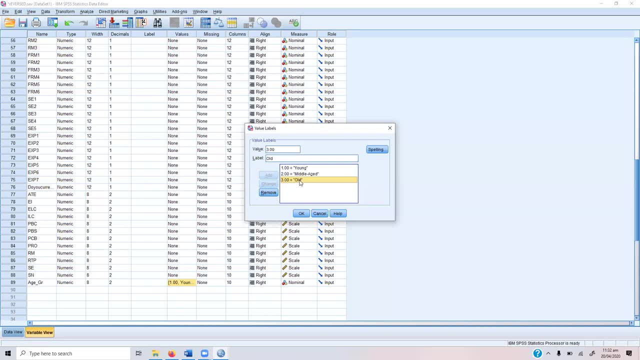 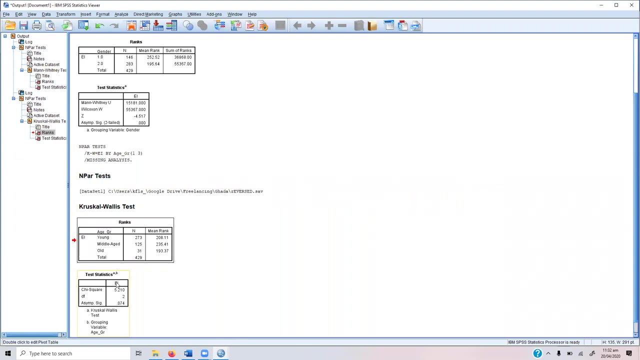 And this actually So the. So our data had three groups, with minimum of one and maximum of three, And that's why the range was one, two, three. I hope it clears your question or your confusion. So let's copy these results into our Word document and let's interpret them. 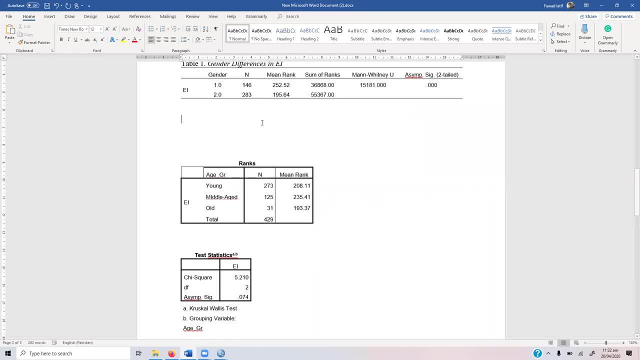 It's more or less the same. Can you turn off your mic, please, And let's take the question? Let's take the questions at the end, please. Okay, Here is our second hypothesis. There are significant differences in EI across different age groups. 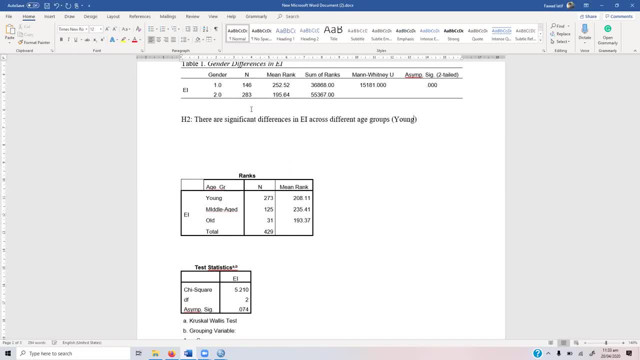 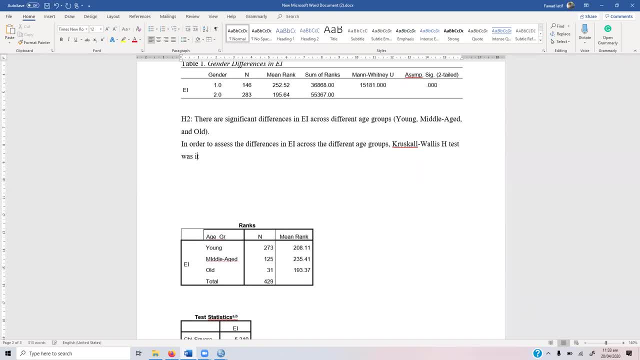 Skull-Boris age test. Skull-Boris age test code test was utilized. Age was divided into groups, namely young, middle-aged and old gold. Now the results are revealed and overall partially significant. why am i saying it's partially significant? 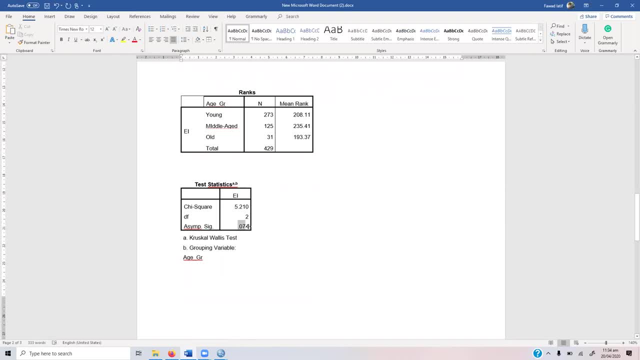 because the significance value is 0.074. now this is not greater than 0.10 and it's slightly over 0.05. so you you should not actually reject your hypothesis in totality, so you can say, have a cautious interpretation and say it's partially significant. 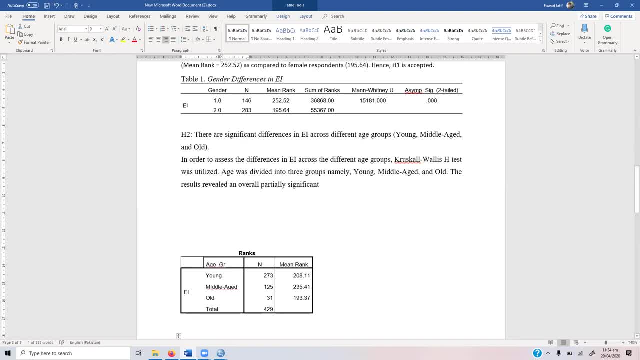 so kruskal had 1l. so i'm correcting my mistake. okay, partially significant, so you can say: or let me put it up. okay, so i square value is 5.210 in the degrees of freedom. here as well, comma e is equal to- now i'm not using less than 0.00 because it's way greater than 0.000, so 0.074. 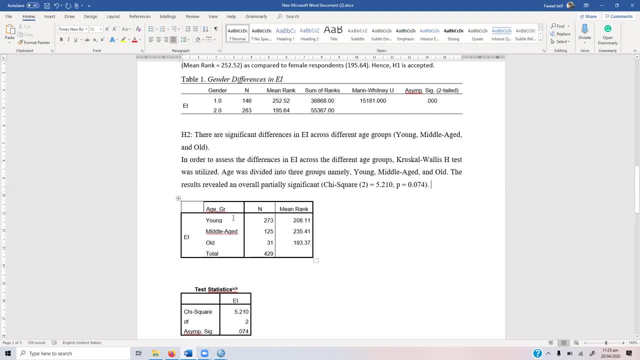 now the next part is: who had the most higher entrepreneurial intentions? mean rank analysis revealed middle-aged employees or respondents. rather than employees, i think it should be respondent highest ei. so their ei was rank is equal to 235.41, in comparison to young rank equal to 208.11 and old 193, sorry, 0.37. 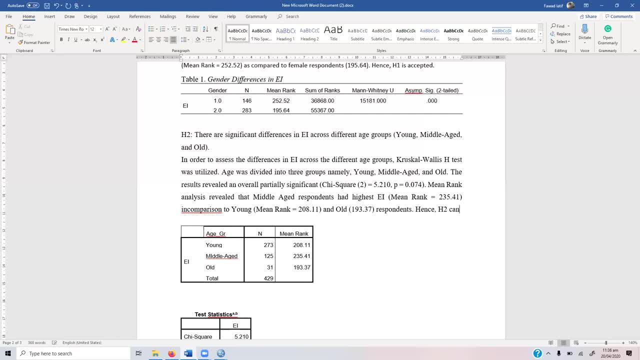 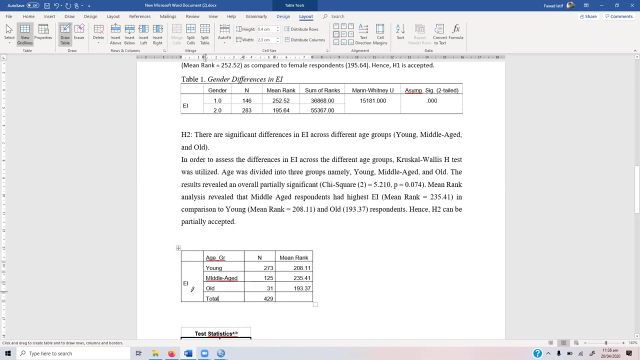 since h2 can be partially now. how do you report the results? let's report the results. format it so a нашем as 2017, 2017. just remove the borders and um it will be. just remove the borders and um it will be. just remove the borders and um it will be. 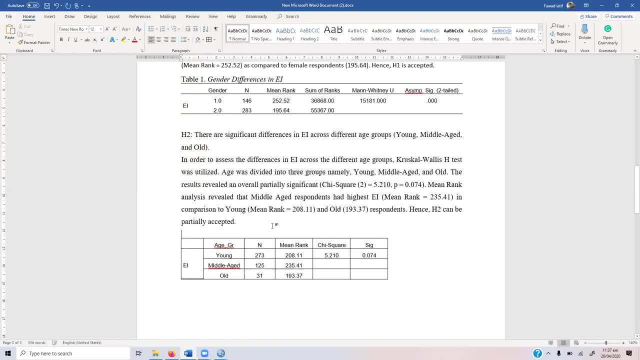 I hope now it's clear how to use Kruskal-Wallis test for comparison across multiple groups and report the results. Now, if you've got any questions, you may ask and we'll. if not, we'll go to our last topic of regression analysis for today, or let's take the questions right at the end, after we've done our. 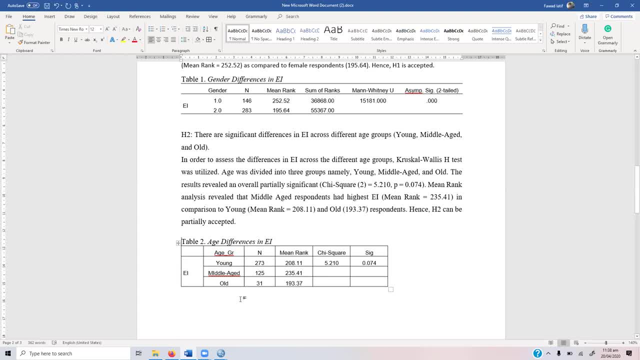 regression analysis as well. Okay, now let's do regression analysis. Now, what is regression analysis or what is a regression? Regression is an analysis technique or analytical technique that is used to identify, evaluate or assess that how much different, how much variation, how much change in a dependent variable is being brought up or brought about or caused by. 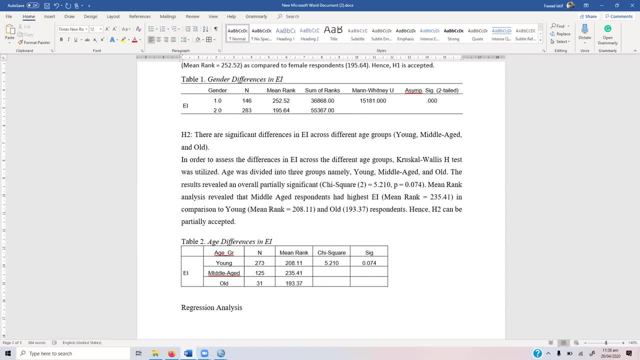 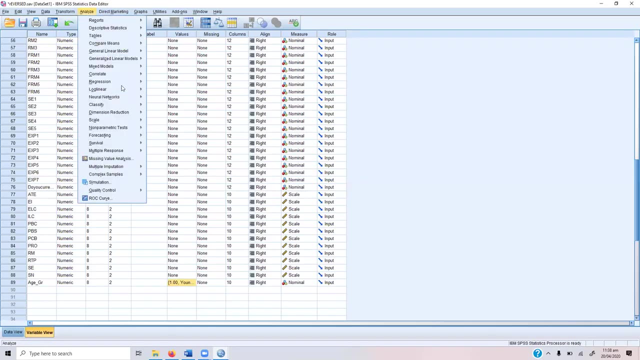 an independent or set of independent variables, maybe one or more independent variables Now. so in order to do this in SPSS, what we do is we go for analyze, regression and linear. So let's say, I am interested in finding out how much change in entrepreneurial intention is brought up by self-efficacy and 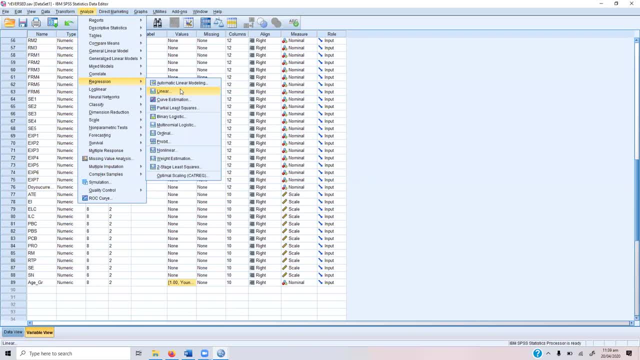 subjective norms or may be internal locus of control or external locus of control. So let's do a simple linear regression in which we have only one independent variable and one dependent variable, and we are interested in finding finding out how much change in a particular dependent variable is being caused by one. 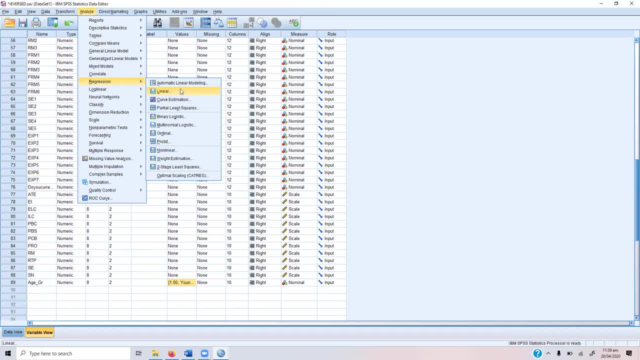 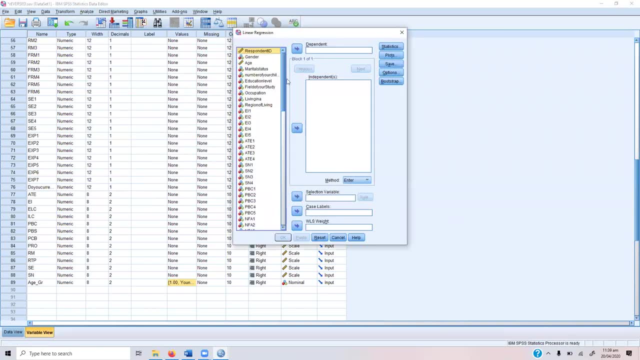 independent variable. so what we do is we go to analyze regression and then linear. so what you do is: i'm interested in entrepreneurial intentions as my dependent variable and my, let's say, self-efficacy as my independent variable. do not need to do anything else, just. 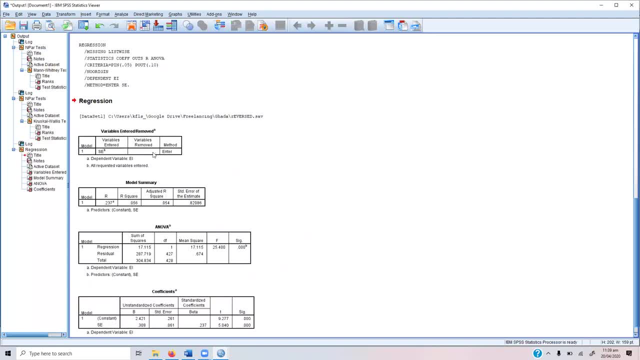 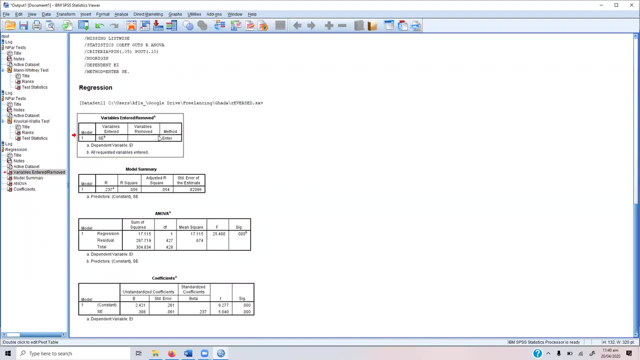 press ok and here you are with your results. you are presented with four tables: one, two, three, four. in the first table, variables entered and removed. what you see is that, okay, this is only the one model that we are testing. variables entered, so you see your independent variable. 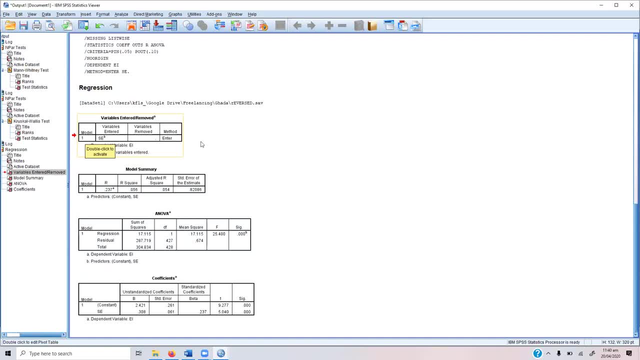 states that i have four variables. i have three variables. i have four variables, i have three here. variables removed. method enter: so since we are doing a simple linear regression, so there are no variables removed, if we were doing, uh, stepwise, maybe forward or backward regression, uh, we do. 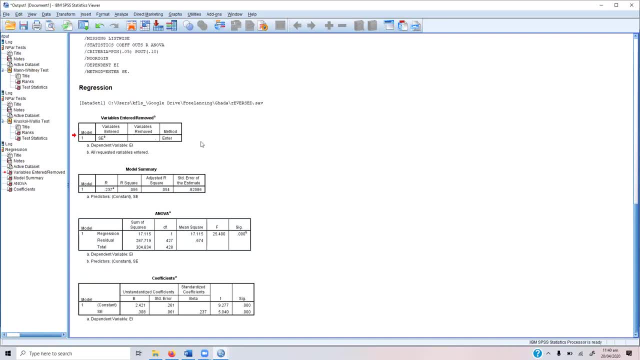 i hope we can meet sometime soon. uh, we can have that as well. or if, uh, i can produce a video on the three, i'll do that, and obviously that will be shared on the channel now. then there is model summary. now what this tells us: that our dependent variable is ei, so correct, uh, and our independent 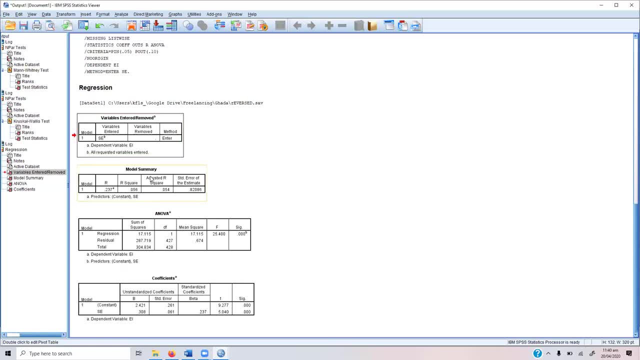 variable is self-efficacy, correct. what's the model summary? now, if we look into it, our model- we have got only one model. so what is r? this is the correlation between self-efficacy and entrepreneurial orientation intention. so r is actually showing us the correlation between these. 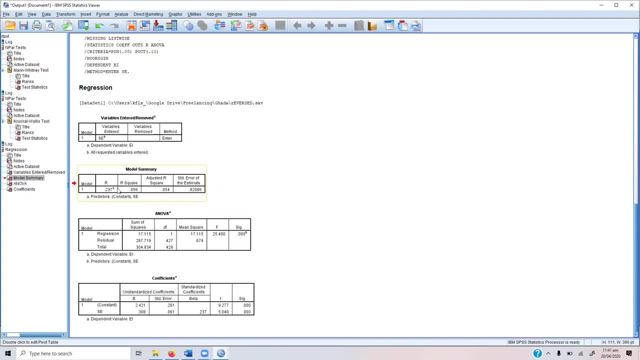 two variables and this shows that it's a weak correlation. the next is: what we are interested in in this table is r square. so if you, if you take square of r, that is 0.237, what you get is 0.056. now what this 0.056 means is that 5.6 percent. if you change, if you multiply by- uh, multiply this. 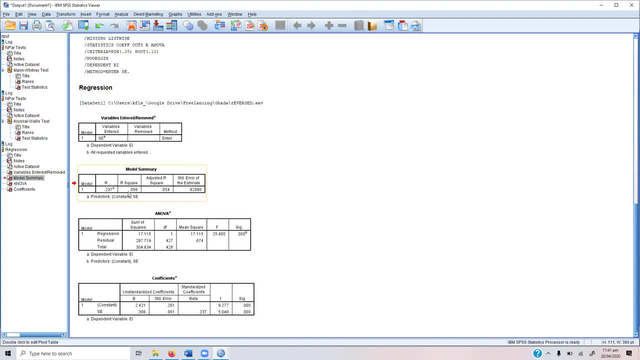 value by 100, you get a percentage. this is called coefficient of determination. so this shows that 5.6 percent change or variation in entrepreneurial intention is being brought up by self-efficacy. so 5.6 percent change in entrepreneurial intentions can be attributed to self-efficacy. 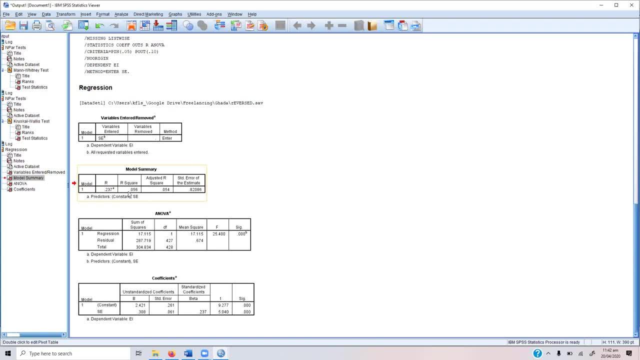 now, is this change significant? is it, is this change significant, worthwhile of studying in our, our research? the? the answer is provided by the next table. if you look at significance, it's 0.000. this shows, yes, the impact of the influence of self-efficacy on entrepreneurial intention is significant. 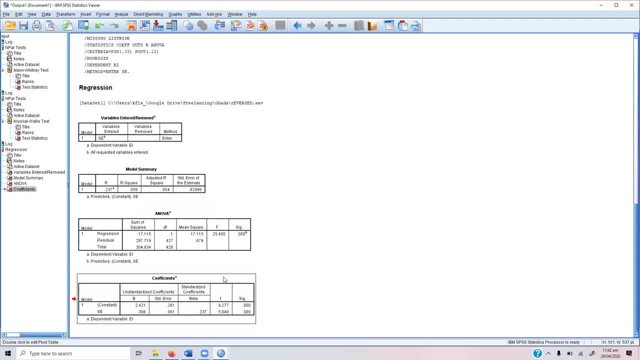 the next table is: is not that, uh, usable in case of simple linear regression? but what if we have got multiple predictors? if so, then as a ret Part Definition in your natural function, when we look at this table and in this in the in the next analysis, we will be discussing this table in greater detail, for 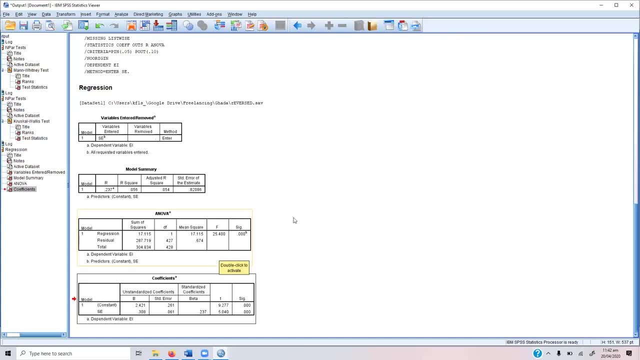 now let's focus on these three tables. so this is how you run simple linear regression and this is how the regression analysis can be easily interpreted. now how to report it. i will do it with multiple regression. so let's run a multiple regression and see how multiple regression works. 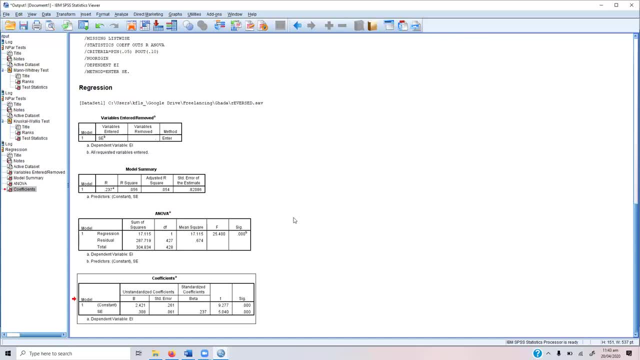 what if there are more than one predictors? what if we have more than one independent variable? what if we have more than one exogenous variables? so, and we want to assess how these variables influence the dependent variable, how these variables bring a change in the dependent variable. so, in order to run, 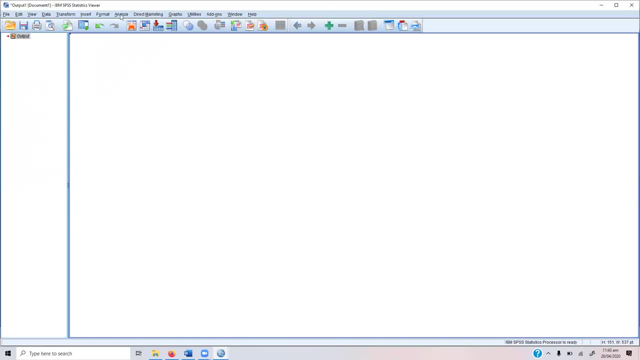 that regression. what we do is we go to analyze regression, and again linear, but this is multiple linear regression now. so, instead of just focusing on self efficacy, now I want to focus on subjective norms as well. now I want to focus on, say, propensity to act as well, and then nothing else, just press ok now. 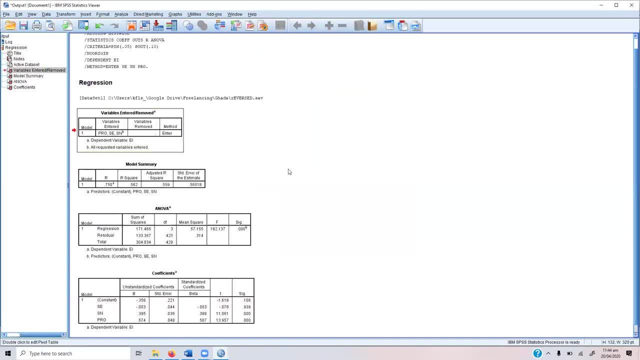 here. okay, have I done it correctly? yes, the independent variables were correctly entered. the dependent variable is correct because the independent variables were propensity to act, self-efficacy and subjective norms. the dependent variable is entrepreneurial intentions. the model summary, now the correlation: the overall correlation between these variable is 0.750 and the R square value is 0.562. so what this R? 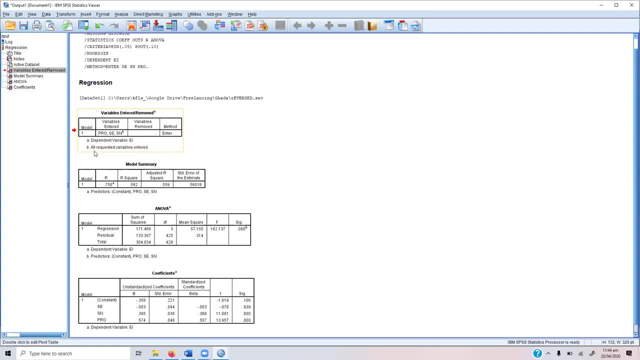 square is telling us is that the independent variables are correct and the way in which we should. Are all these three variables significant? So I'm asking you this question: Whether propensity to act is significantly influencing, self-efficacy significantly influencing and subjective norms significantly influencing. 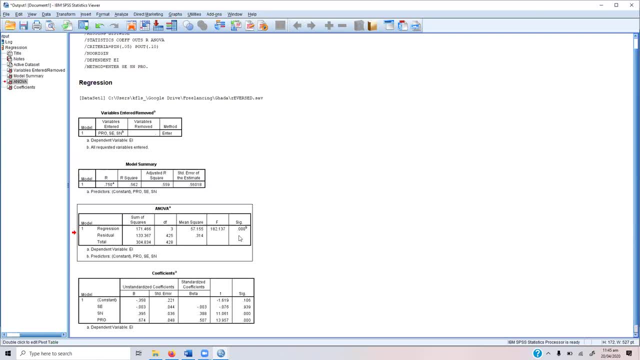 So now, how do you answer this question? In order to answer this question, whether or not each one of them is significant or not- you go to the coefficients table And if you look at this table, under constant, you see self-efficacy. 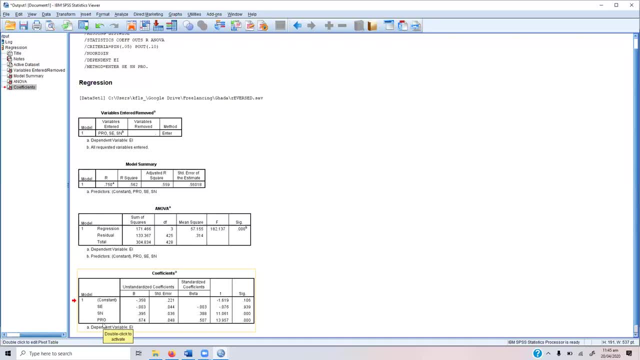 subjective norms and propensity to act And their beta value, their weight of impact. their weight of influence, how much weight they carry in influencing the dependent variable. It should be over 0.20 in order for it to be significant, But sometimes, even if it's less, it's significant. 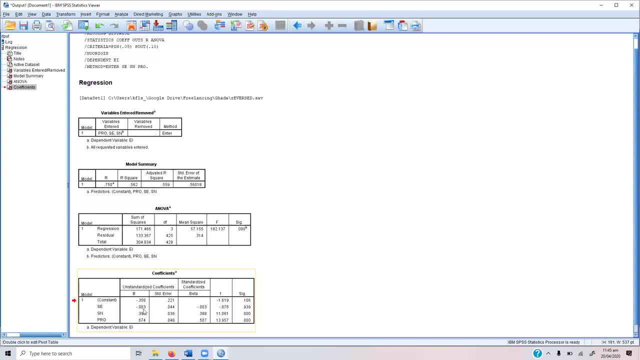 In this case, if you see self-efficacy- self-efficacy which was previously significant in our last analysis. now it has suddenly turned into insignificant. Now this is a very important thing. How come a variable which was significant individually 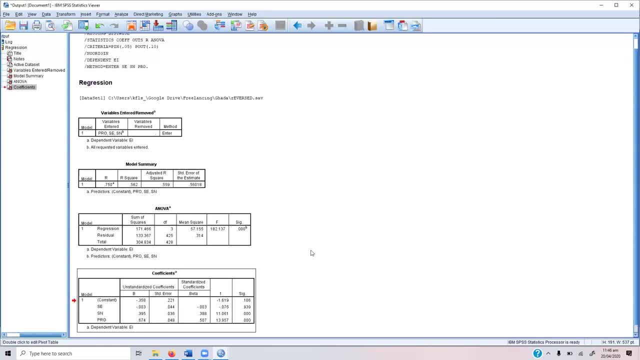 becomes insignificant when you have got multiple regression. This is pretty normal And this happens in. let me give you a more plain and simple example. For instance, you are pushing a car And you are trying to push a car If somebody weighs around 70 or 80 kg. 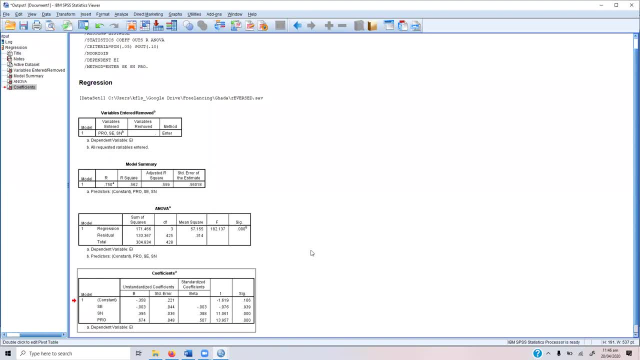 he might be pushing a car and it's just like slightly moving from its space Or its place. Suddenly, a person comes and he's a bodybuilder, a very Hulk-like man, And he starts to push the car. Now he will be able to take a car much further. 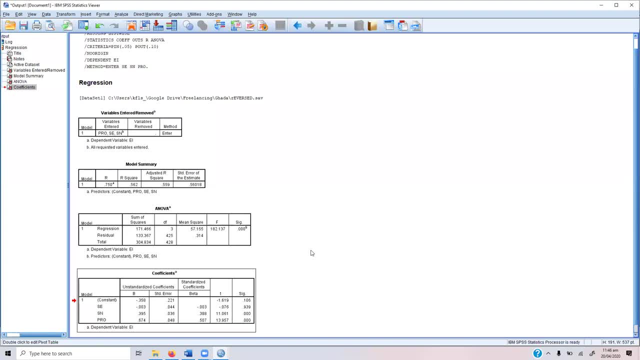 than what a 60 or 70 kg man was going to put it or like move it. So when the Hulk man like comes, his impact is far greater than the other person And that person who weighed 70 or 60 kgs. 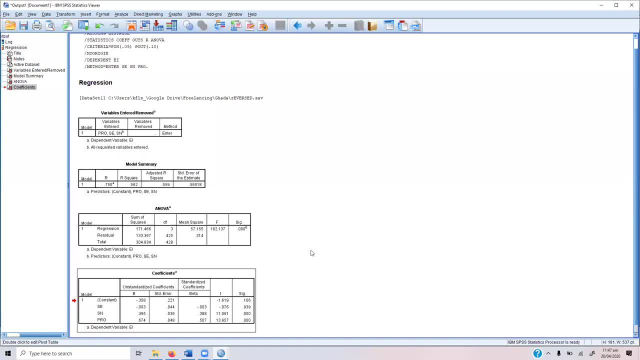 his impact actually diminishes or it finishes. This happens in regression analysis as well. With the entrance, with the advent of another variable, the impact of the other variable might diminish to an extent that it becomes insignificant, And this is what happened in this case. 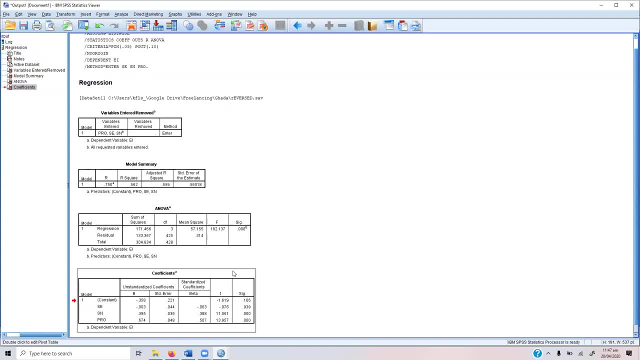 While self-efficacy individually was significant, But with the advent of propensity and subjective norms, its influence in the organization or within the respondents becomes insignificant. or it became insignificant How do I know it's insignificant? Because the significance value is greater than 0.05.. 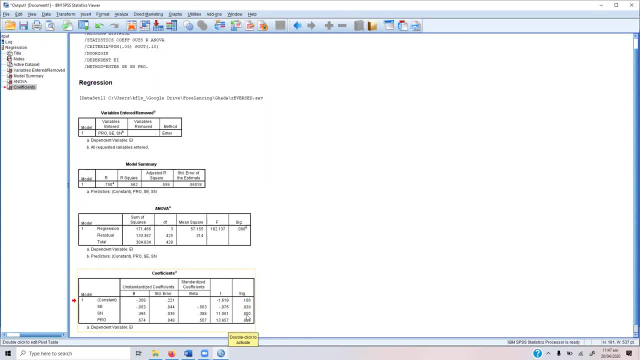 While for the rest of them- SN and propensity to act- it was significant less than 0.05.. The T value for self-efficacy is less than 1.96.. While for subjective norms and propensity to act, it is greater than 1.96.. 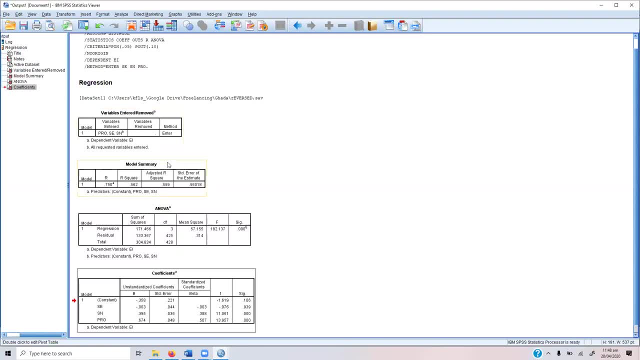 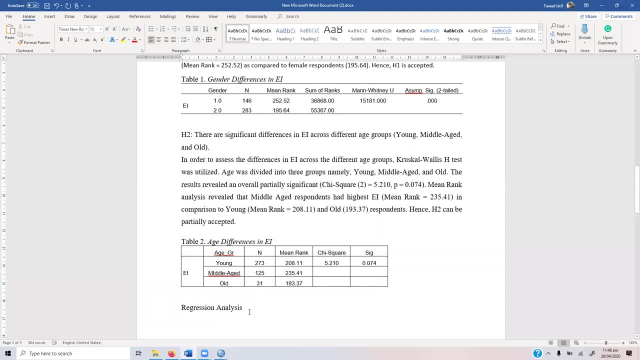 Now, how do I interpret these results? I do not need my first table, I only need these three tables, and let's use these three tables to interpret our results. Let's go for regression analysis and let's put it in a separate page. 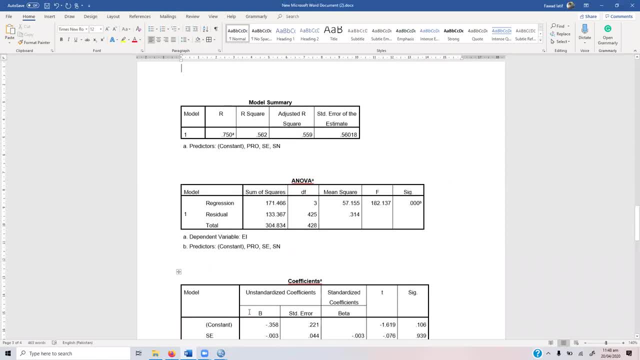 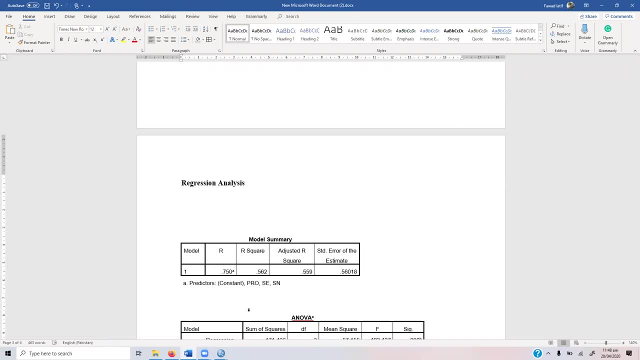 Let's propose our hypothesis. Let's say H3.. Here is a significant impact of self-efficacy on employee intentions. Let's put it in a single hypothesis. So H3.. A is there is a significant impact of self-efficacy on entrepreneurial intentions. 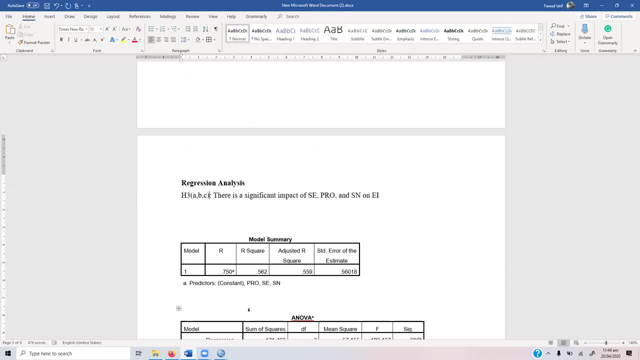 H3B is impact of propensity to act on entrepreneurial intentions and H3C is significant impact of subjective norms on entrepreneurial intentions. Let's propose our hypothesis. Let's try a low-level hypothesis with prime time learning and theoretical derivations Behind what this difference means. 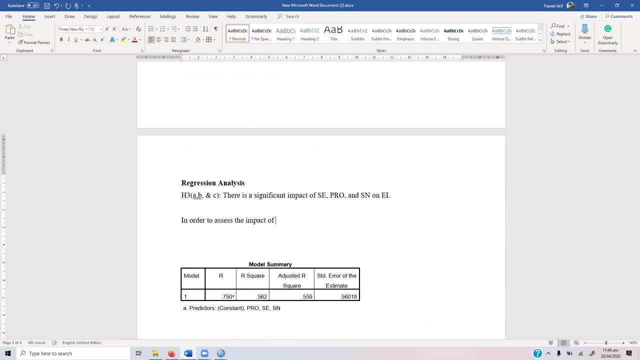 we know that we all need these three tables, so we can argue for There is a difference between H3 and B. We backtrack to our aim and we look for. Part of this question was focused on ensuring this network between four-year time management and three-year time management agreement. 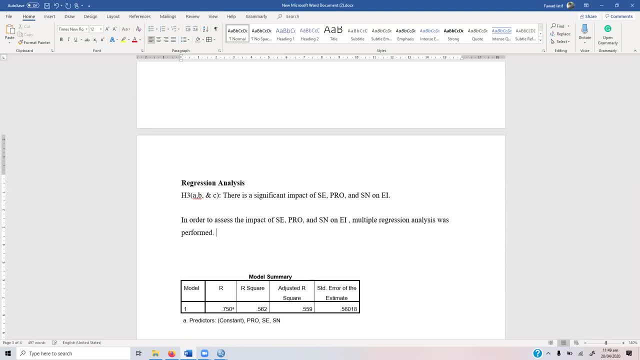 I will first ask one more question. I'm making an in-depth medical calcчно oosy here. The unit where three, four, five modules are included, 제1. These would be abut two weeks of epi, summary section ،. 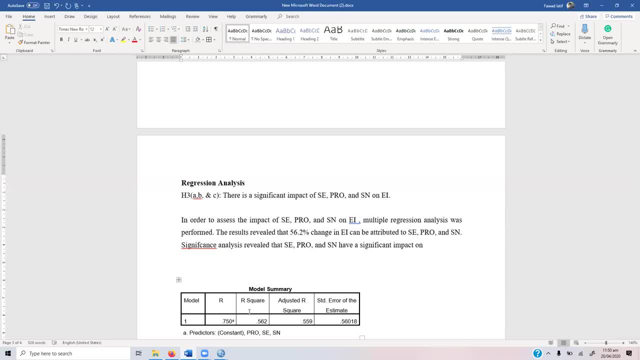 report the F value where this 3 is from here the degrees of freedom, and then comma the residuals. and then what we do is we write 425 here and the P value is 182.137. comma P value is less than 0.001. now, this one's done. let the end. so we can interpret the law. the other table as: 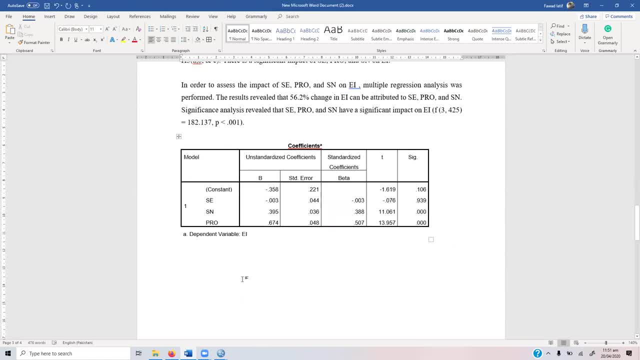 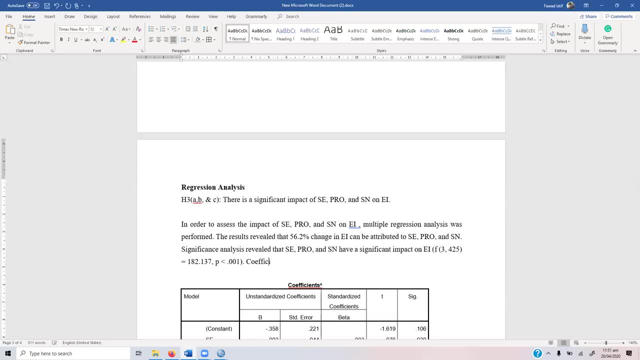 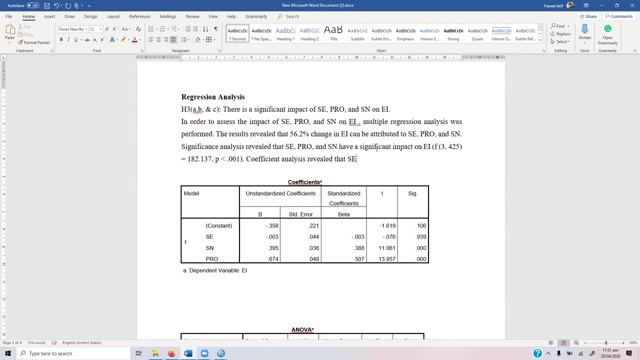 well, what does the coefficient table tell us about the impact of each of the individual variables? so coefficient analysis revealed that- let's make the whole table visible- that SC did not succeed significantly. and then you write: D is equal to 1076. one more thing: it's always. 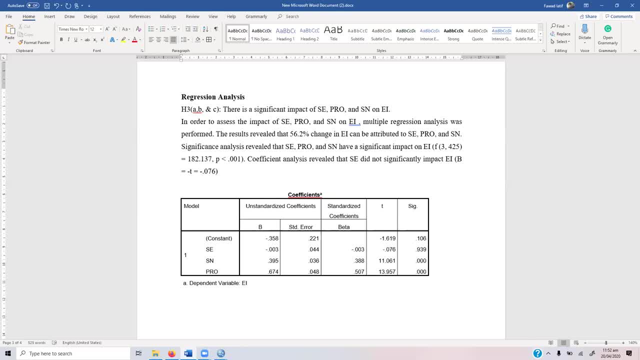 a good idea to report your beta value, which is minus 0.03, and your E value is equal to 0.939. 3A was Okay, Let's do the next one: SN. SN had a significant impact on BI, so you report those results. 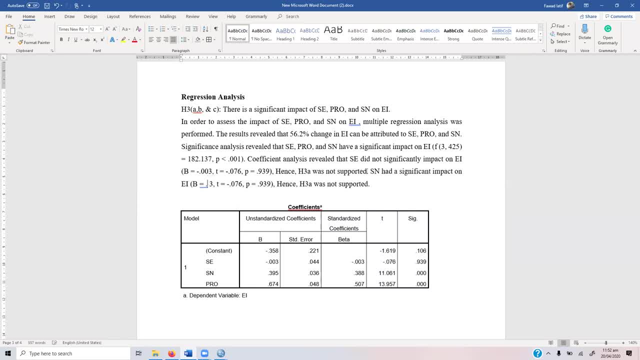 as well. Beta is equal to 0.395, T is equal to 11.061 and P is less than 0.001.. H3B was supported. Let's do the last one, which is propensity to act. It's always advisable. 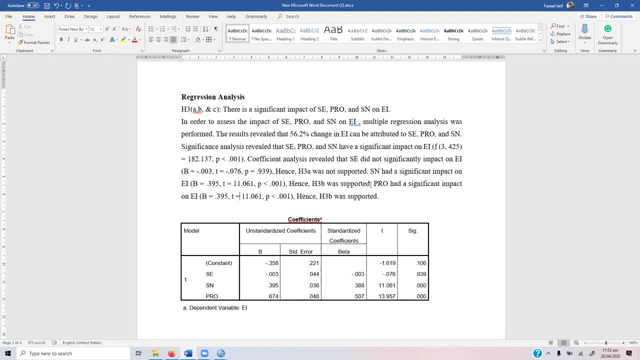 to write the full form. as I mentioned in the last analysis, Beta is 0.674,, T is 13.957 and H3C was supported. Now let's arrange the results in a more meaningful way. Let's make it a full border and 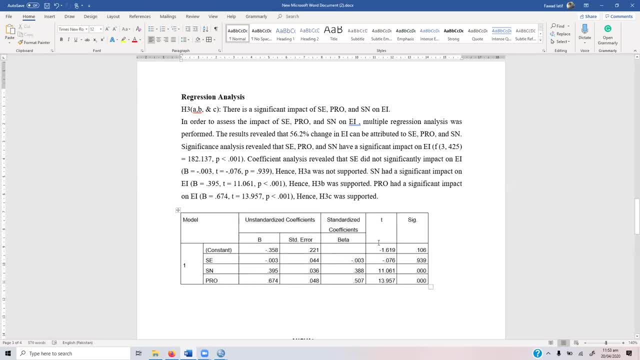